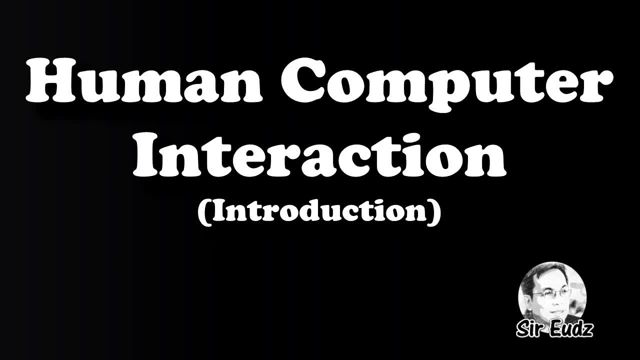 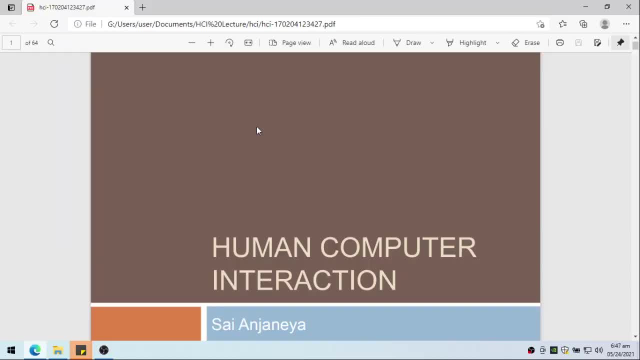 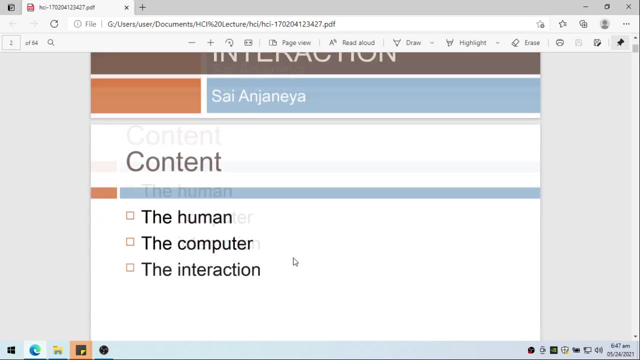 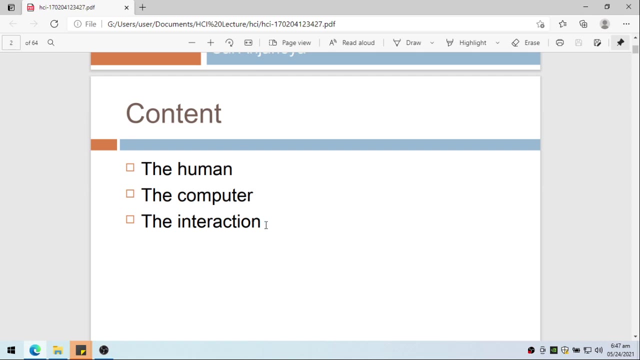 Today I'll be introducing to you human computer interaction, and I'm using the slide made by Sai and Janaya. I hope I pronounced correctly, so the contents of the introduction will be the human or the contents of this slide will be the human, the computer and the interaction. but this will be the first part of the. 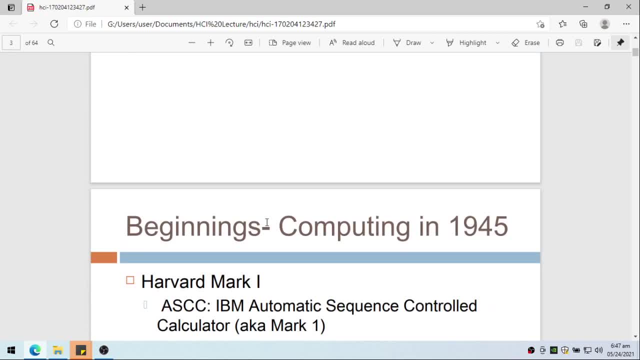 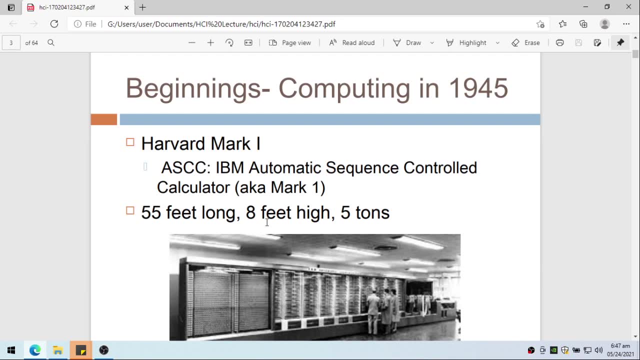 series of videos. now to understand human computer interaction, let us first take a look at some some sort of history of the computers, so the beginnings of computing in the year 1945. so in the year 1945 we have these computers, the Harvard mark 1, so as shown in the picture. so IBM automatic sequence. 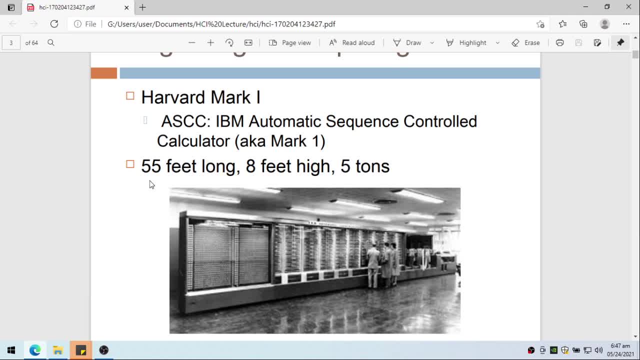 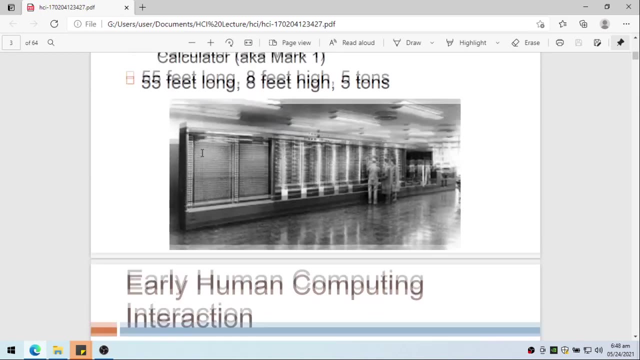 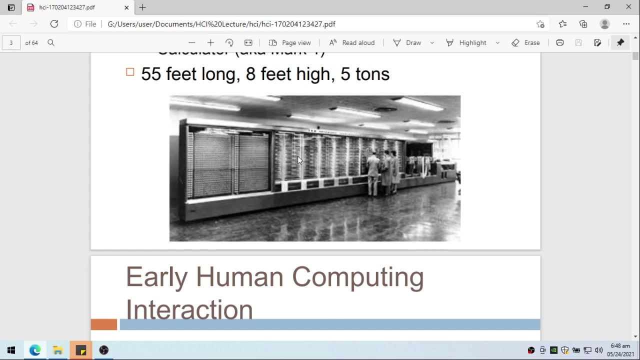 controlled calculation calculator, also known as mark 1, and the size is 55 feet long, 8 feet high and it weighs 5 tons. so that's how big this computer is. and you know, this is just a calculator and maybe, if we, if we're going to look closely at the picture, you can see how 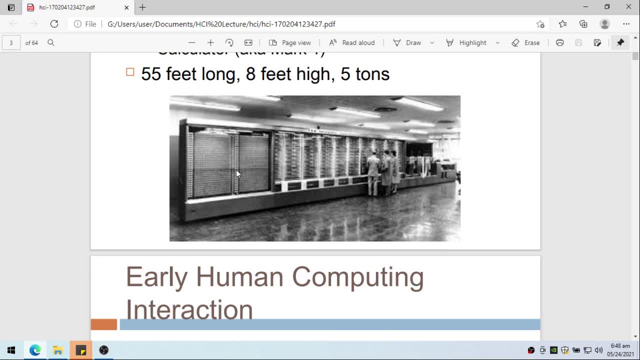 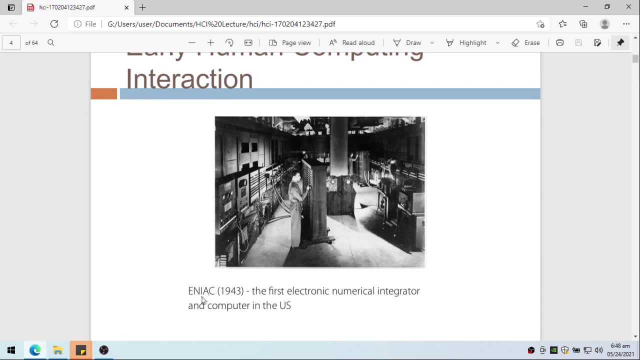 complex it is. so this is a computer or a calculator. then here we have another computer. we have the ENIAC 1943, the first electronic numerical integrator and computer in the US, and you can see also the how this computer looks like. so we have a lot of switches each other, and they are so. 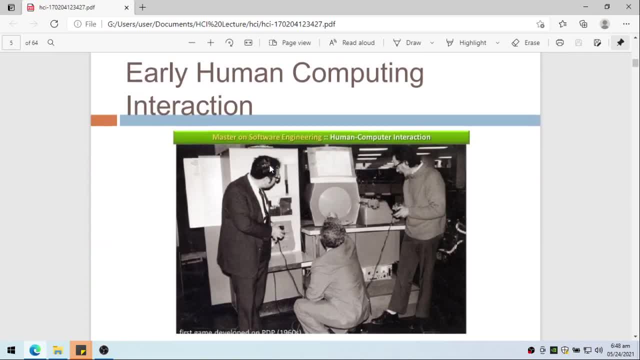 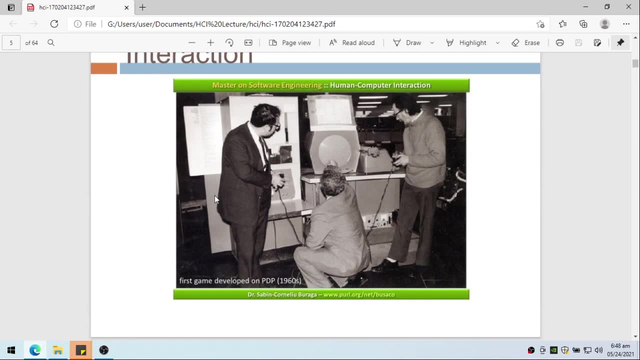 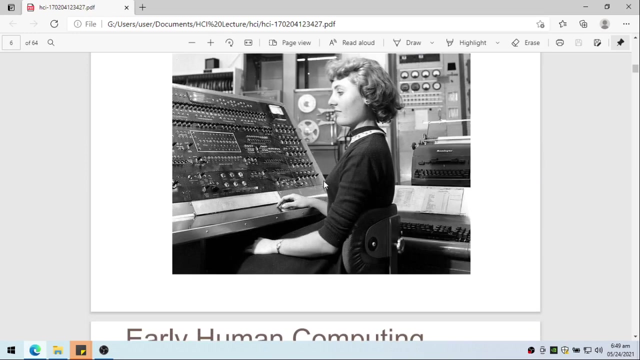 quite so big. here is another one. this is the first game that was developed in the 1960s on PDP during the 1960s. so again we're using some sort of a big machine. then here is another computer during the, the early days. so just take note of the. 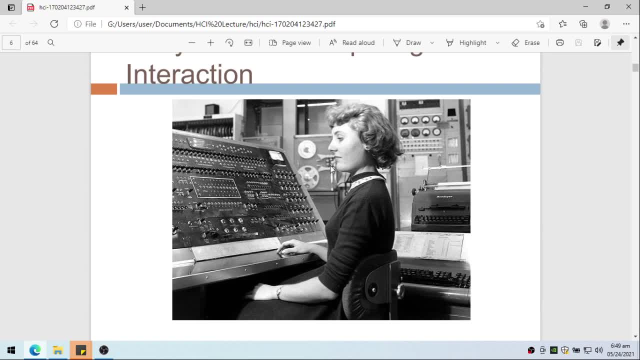 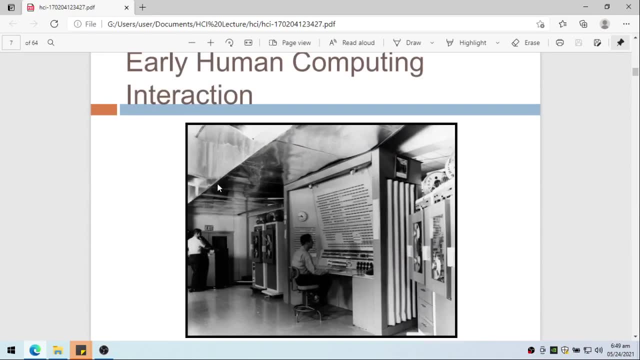 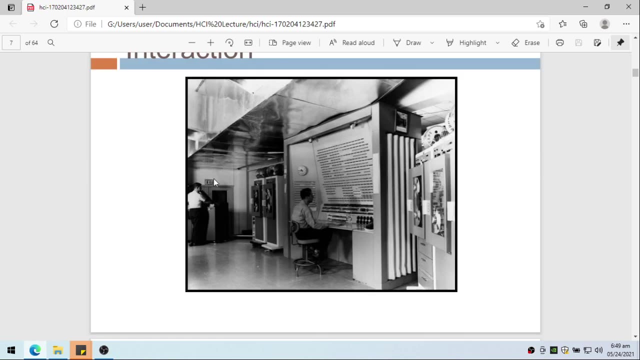 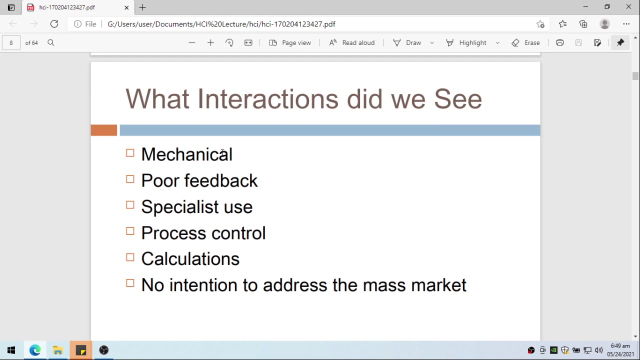 panel and take a look at the more or less these devices here. here's another machine during those years, the early years of computing, and what have we observed? so what interactions did we see? we can see that the interaction between the human and the computer is quite mechanical, so there are a lot of switches, and maybe we can say: 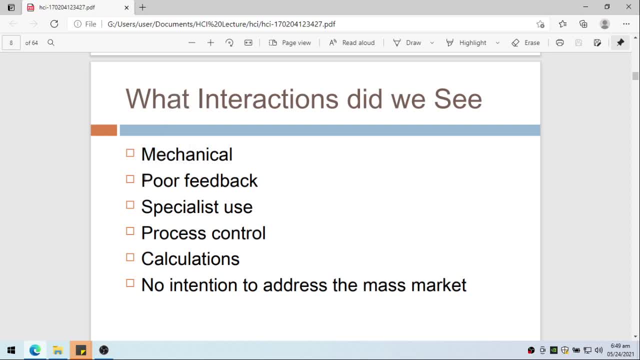 that there's poor feedback because, uh, there are. no, we have, uh, we have big machines, but there are only few monitors to give us some sort of feedback or output, and we can say that this is not for everybody the first place. who can afford to have a computer that big in their own homes? or 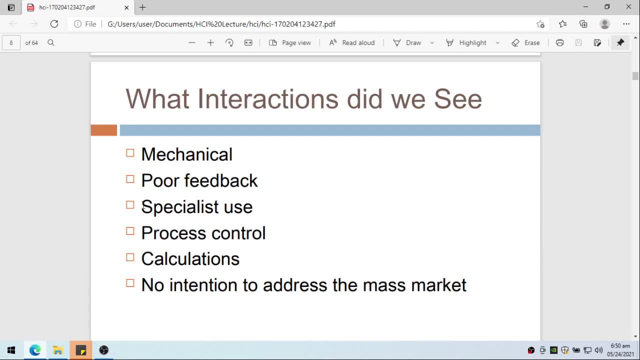 and who can actually place those computers in your pocket. so the computers during those days are only used by specialists, so those who are trained to make use of the computer. so we also have process control calculations. so these are more or less the things that are being done with the computer. and then, of course, just like what i've said a while ago, there's no intention. 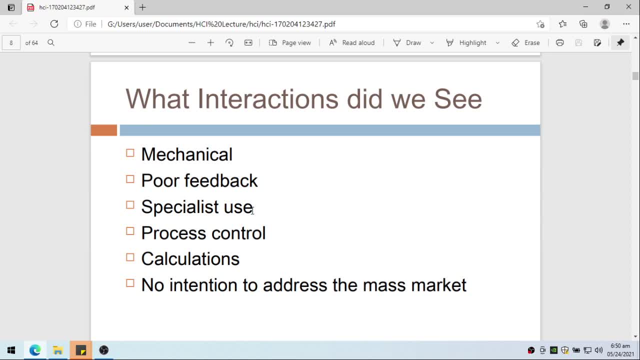 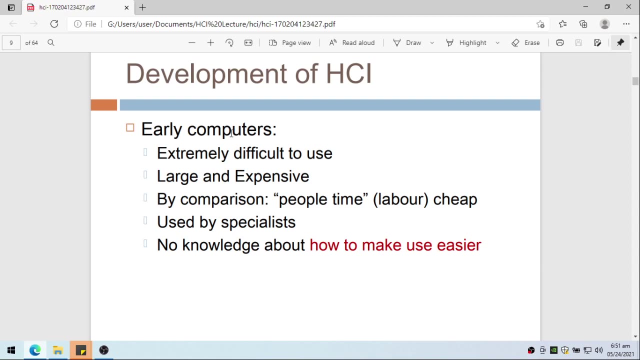 to address the mass market. so these are only used by specialists and, of course, it was used by big businesses during those days. now the development of hci. so let's again take a look at what we have seen a while ago. so the early computers are extremely difficult to use because, as we have said, 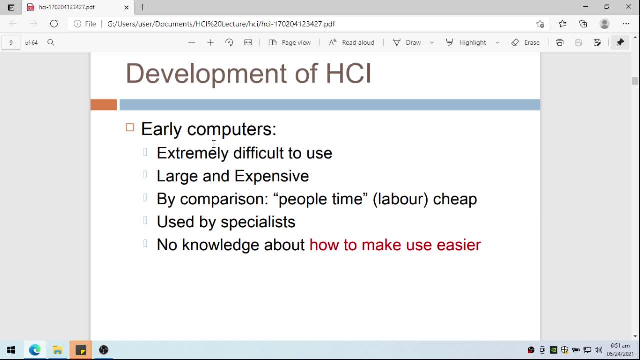 it needs specialists to make use of this computer and they're large and expensive. so, by comparison, people time, labor is cheap during those days. so it's used by specialists and no knowledge about how to make the use, how to make use easier. so that's because, of course, 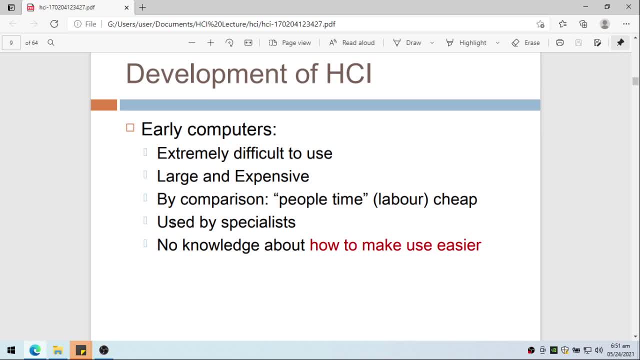 only a few people are using the computers. so whether it's difficult or not, no problem. because it should be only used by specialists and there should be some sort of a training before somebody can use it. so that's why i'm saying it's difficult to make use of this computer. 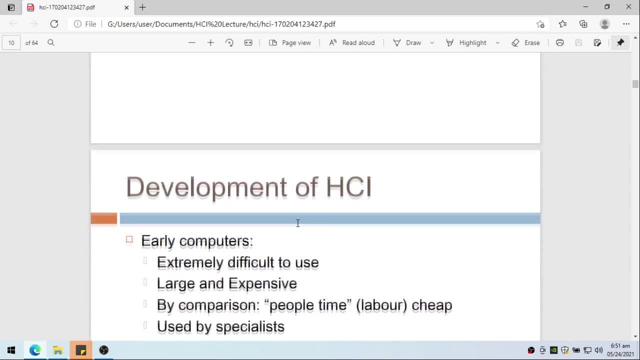 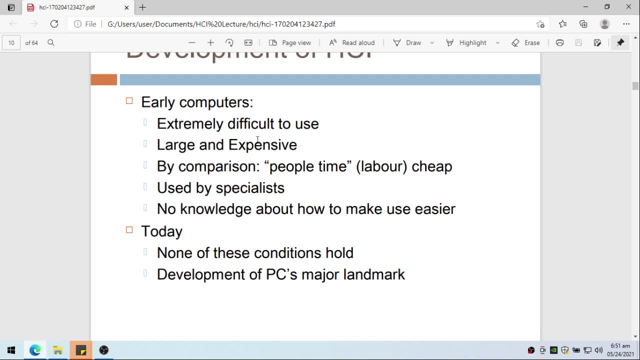 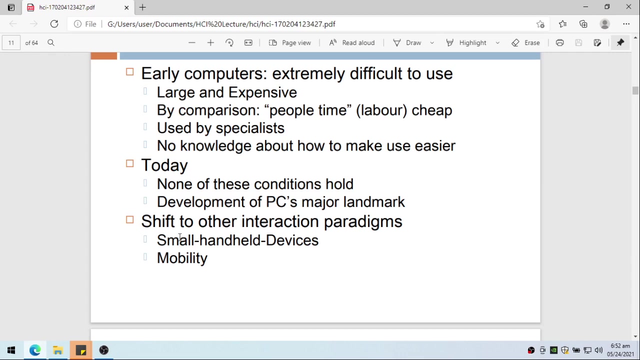 and use these devices. today, none of these conditions already hold, or maybe just, uh, almost none of this. not, not totally not, because one thing is the development of pieces of personal computers, and that's because, and that's the reason why, almost none of this already exists. and then there's a shift to other interaction paradigms. 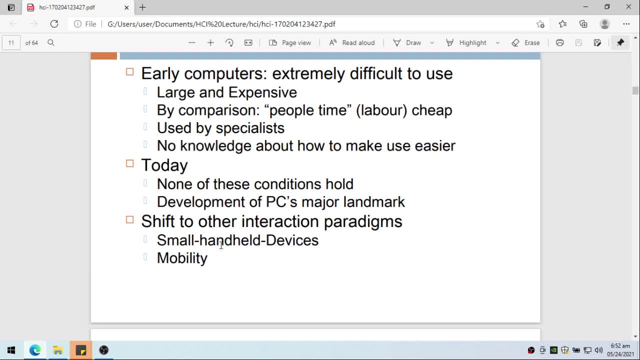 so now we have have small handheld devices like your cell phones, your pdas, and mobility, so we can have our uh. we can just place our cell phones in our pocket, we can. laptops are portable, so we have mobility during those days. as compared with the early computers we're in, they're actually big and large and expensive, so now they are. 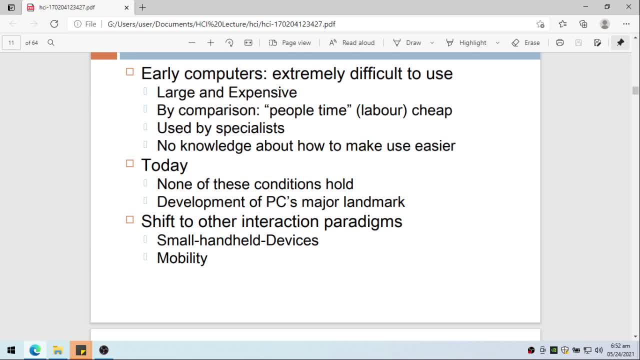 smaller and affordable. that's why more people now can make use of computers, so let's go back to that. so because of that, since more computers now will be making use of computers, and not only by specialists, then it is now a special concern to make this, or to make computers, or maybe the applications used by this computer, easy to use. 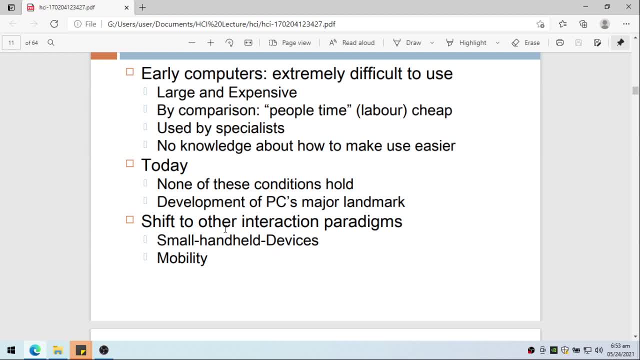 so not only by specialists but by everybody. that's why, as we can see, more or less almost everybody, if not everybody, already have cell phones or most have their laptops at their homes. so, as compared with maybe the early computer, early computers or the early years of computing, 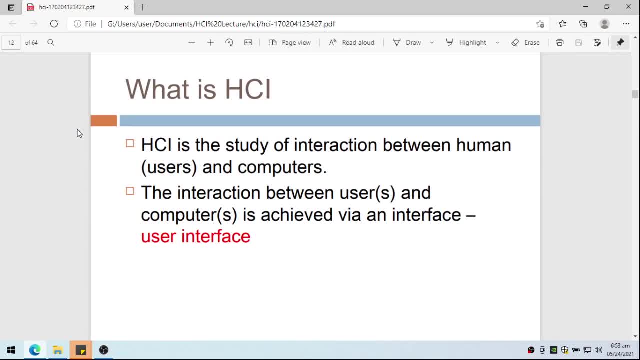 so with that, what is HEI? HEI is the study of interaction between computers and mobile phones. so we can see that this one is HEI between human, or the users and computers. so the interaction between users and computers is achieved via an interface, and usually we call that the user. 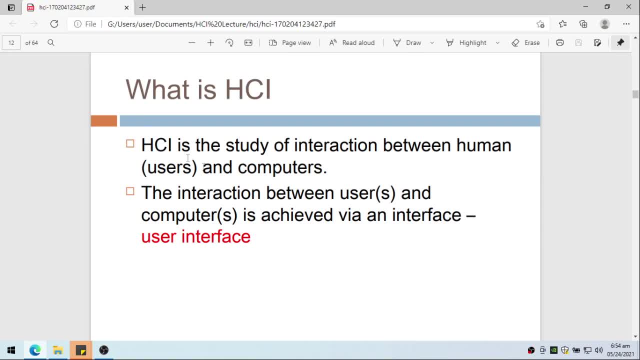 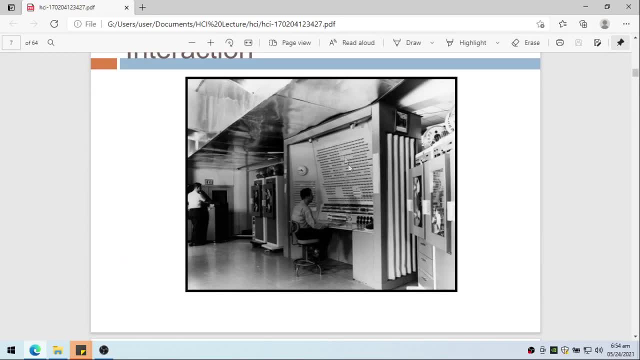 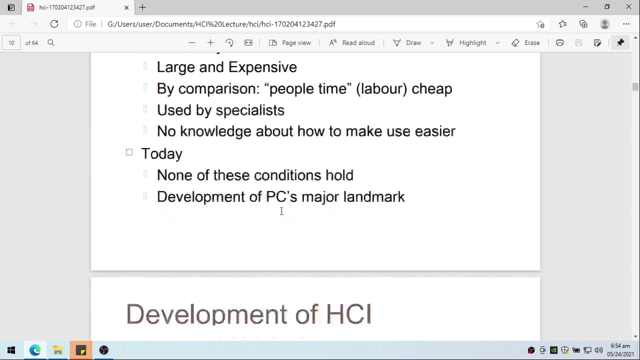 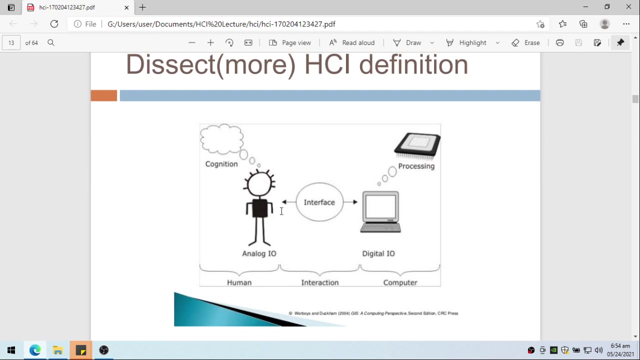 interface. so if you're going to look at, let's take a look at the previous images. so just take a look at the user interface of this computer. it looks like more complex than that of an airplane panel. so let's dissect more of HCI definition. so we have human and this is 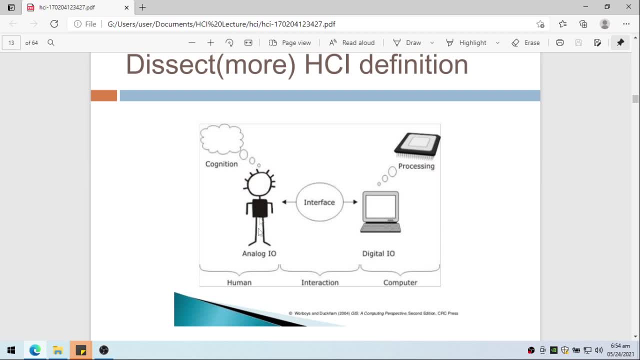 the computer and we could say that human also receives input and it actually thinks using the cognition. and of course the Human will see the user interface or will interact with the computer using the input and output devices. the digital I own and of course the computer is also. 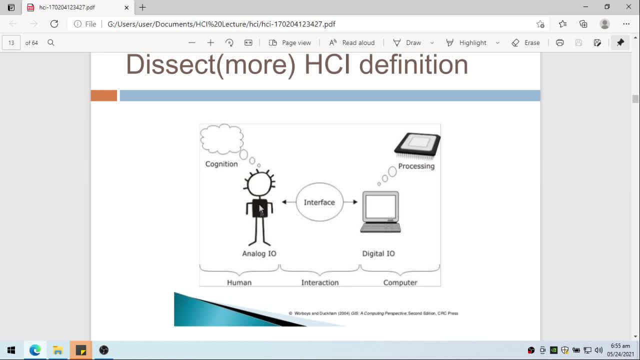 processing those data and the Human now will interact with this by the interface, the user interface. so let's say, for example, the interface says places are the buttons, so the human will click on the buttons or the interface will drive the comment mind. Then the production by cutter device, using the human and the computer together. 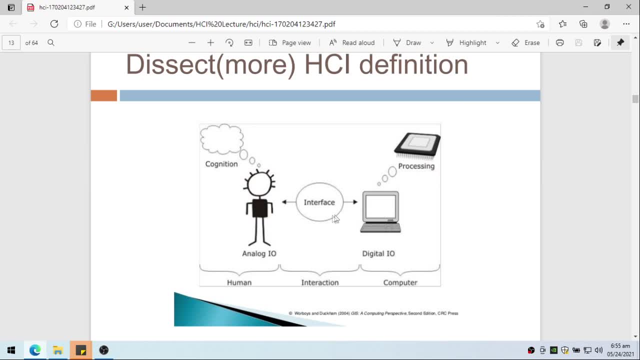 phase says that you enter your name, then the human will enter steam, so that you are. the human now is interacting with the computer, and that's what we call human computer interaction. and of course the human, human's action is of course being controlled by cognition, or the way he thinks. 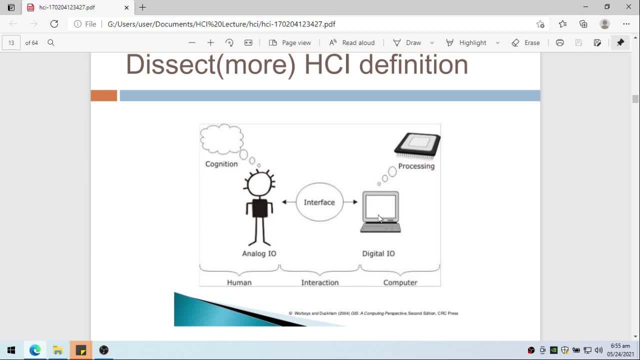 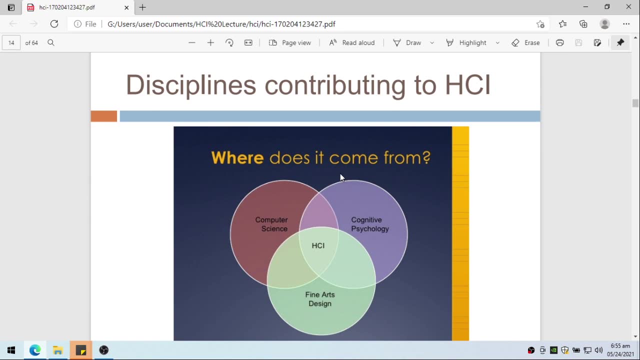 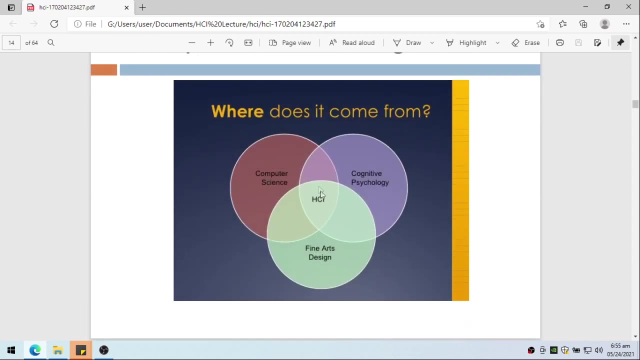 and, of course, a digital computer now process the data using the processor and the application. so this: there are disciplines contributing to hci. so where does it come from? so we have to include computer science technology and we also have to use cognitive psychology. we have to know. 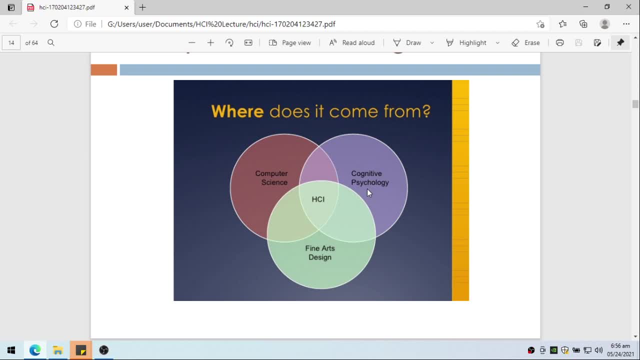 how humans think or how human, let's say, remember things, or how human interact with things, and we also have to make our interface, of course, presentable. so it's an art. so we combine the technology, the human psychology and art and the intersection among these three disciplines.